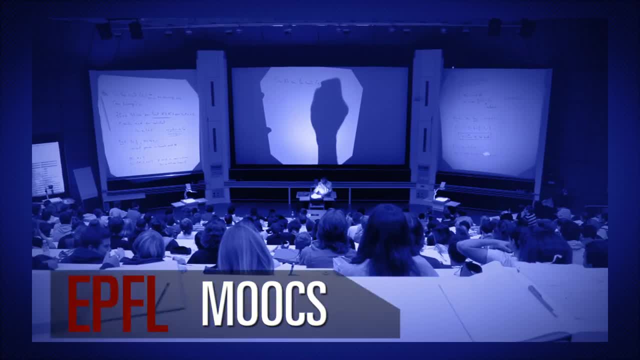 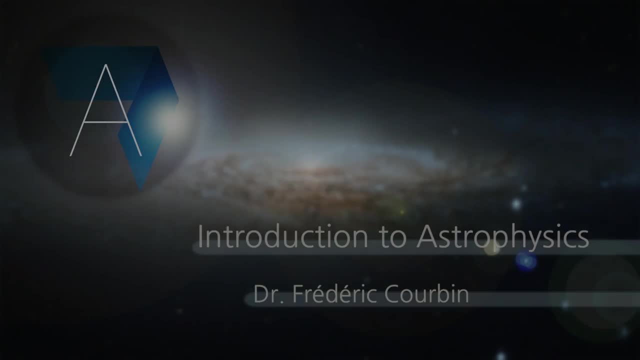 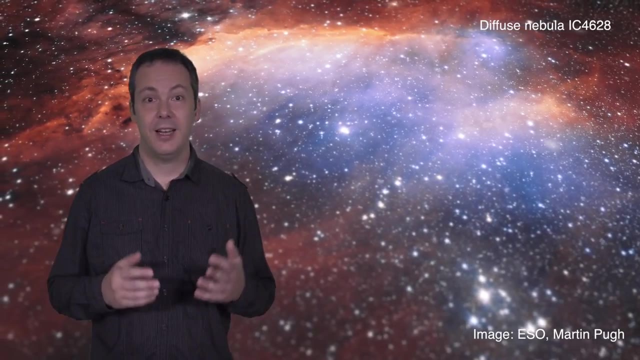 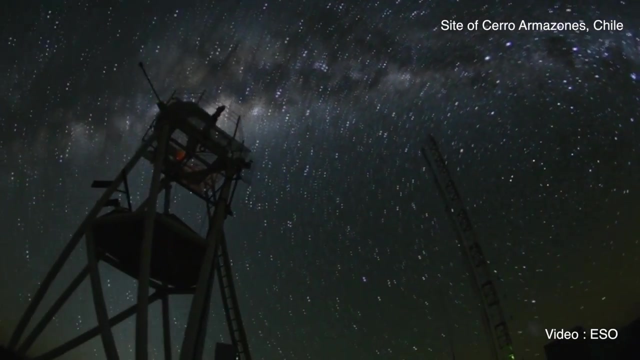 How is the world are we living in? How to study the universe using the only information we receive from it: light. The goal of this course is to provide an overview of the physical concepts used in astrophysics to analyze the observations taken by large ground-based and space telescopes. 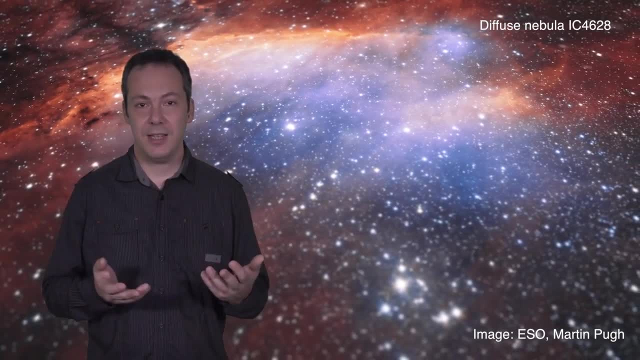 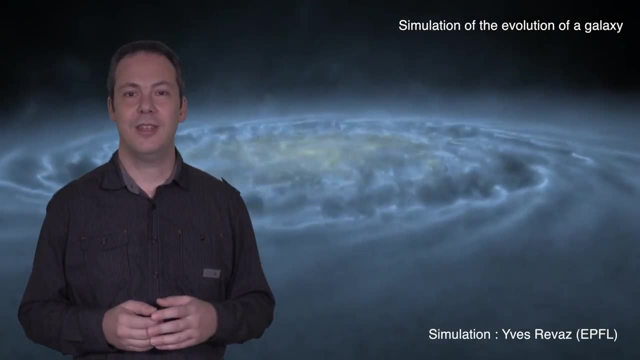 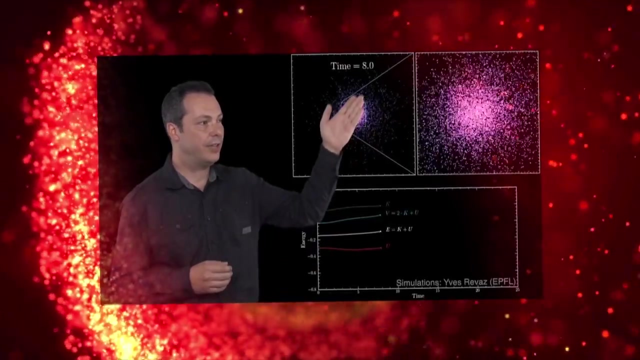 with these observations. the goal is to imagine the physical mechanisms responsible for light radiation we receive from celestial bodies and for their motion, and to model them. and of course, as always in science, one needs to confront theoretical predictions to observations. the material in this course spans a broad range of theoretical concepts, which astrophysical, 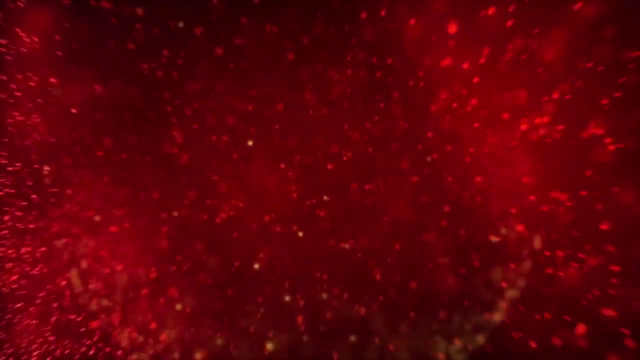 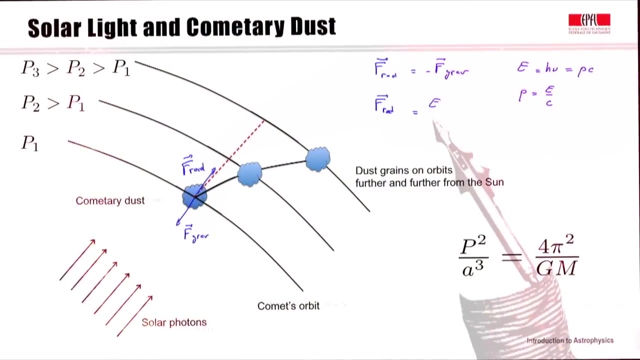 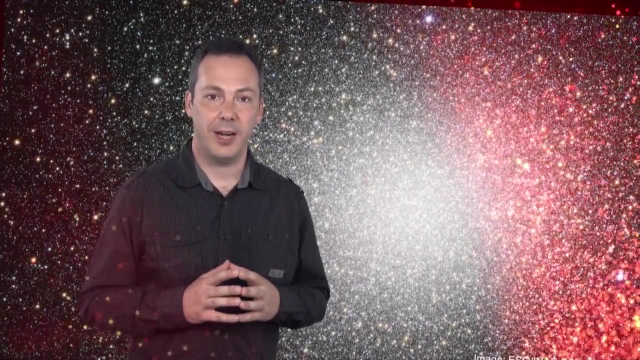 applications play a role at all temporal and spatial scales. the course is organized as a voyage from our solar system to the whole universe, from stellar formation to galaxy evolution. to this end, we will use images, demonstrations on the slide pad, focusing on the links between theoretical concepts and observations. my name is Frederick Corbin. I am a researcher at the laboratory of 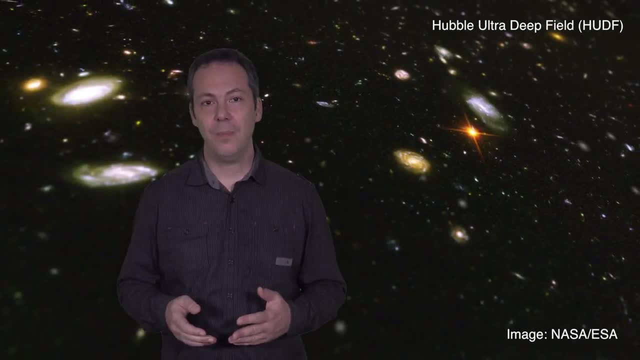 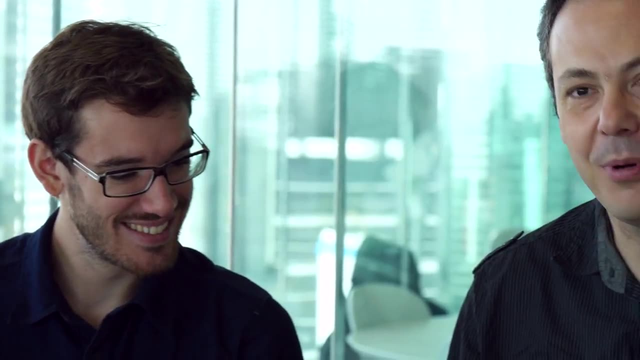 astrophysics of the Swiss Federal Institute of Technology in Luzon, where I split my time between research and observational cosmology and teaching. the course I propose here is given to students who are in physics in their second year bachelor at EPFL. it consists in the mandatory 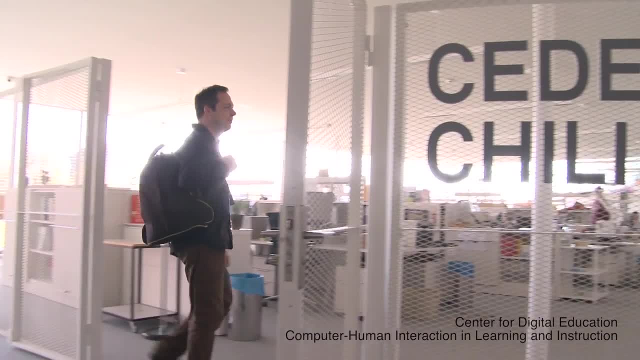 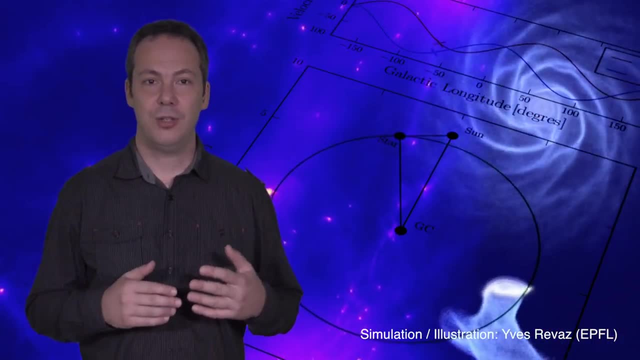 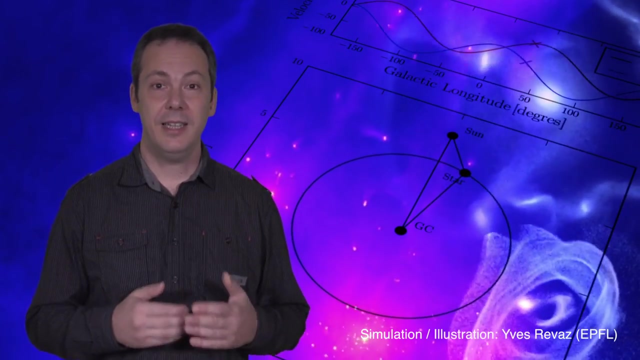 basis for the more advanced astrophysics courses, but also allows students to see physical phenomena they may already know, but in a completely different context. prerequisites are minimal. they correspond to the knowledge of a first year of university. in physics they include trigonometry, simple integral calculus, Taylor expansions and solving first-order differential equations. 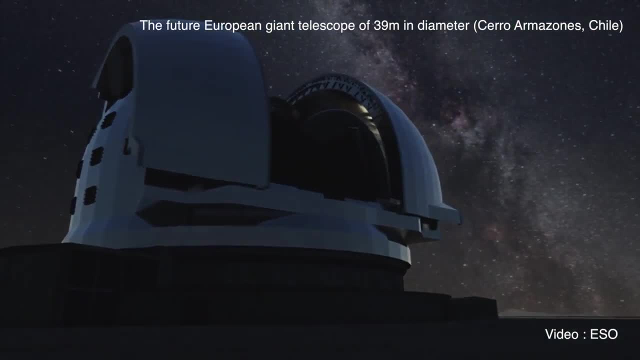 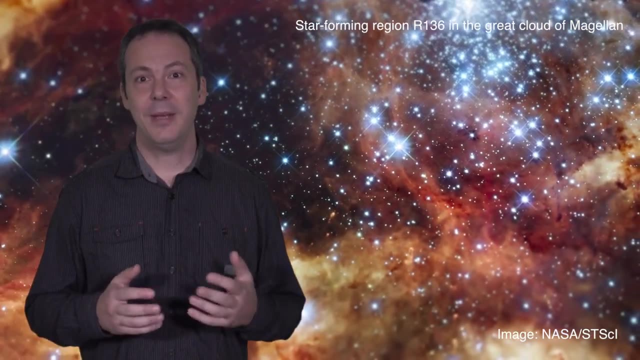 as we put much more emphasis on the physical concepts than on long numerical developments, the course remains simple and accessible to most of you. I am looking forward to meeting you very soon for this introduction to astrophysics.